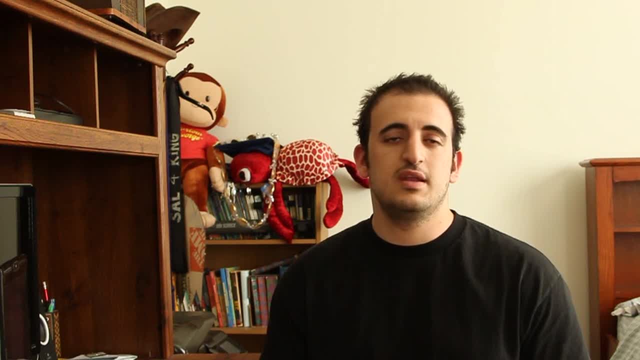 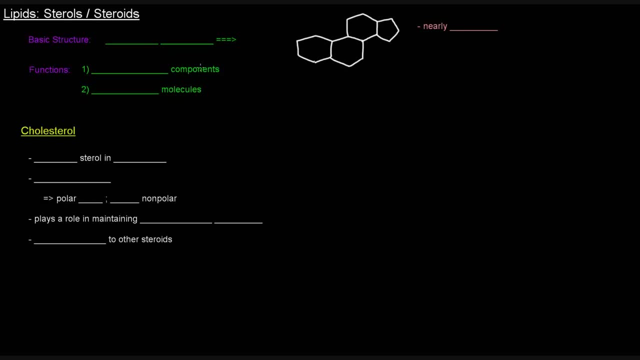 Hey folks, if you'd like to support me or this channel, Moof University, in creating more video tutorials, then please consider making a financial contribution at my website, moofuniversitycom. Thanks and enjoy the video. I'd like to wrap up the discussion of lipids by talking about sterols and steroids. 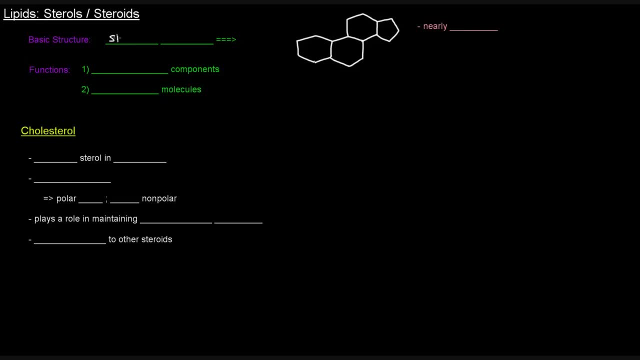 So their basic structure is based on this idea of a steroid nucleus. Steroid nucleus which I've drawn here. It's this four-ring system. Three of them are six-membered rings and this last one is a five-membered ring. 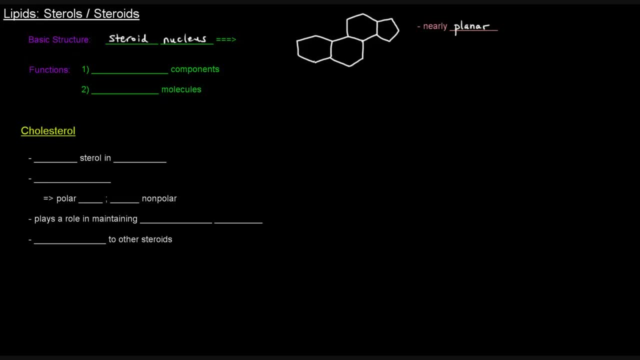 And this whole situation is nearly planar. The rings are referred to as the A-ring, B-ring, C-ring and D-ring Now. so all steroids have this basic structure, this basic four-ring system. They vary slightly from one to the other, but they have that same sort of situation going on. 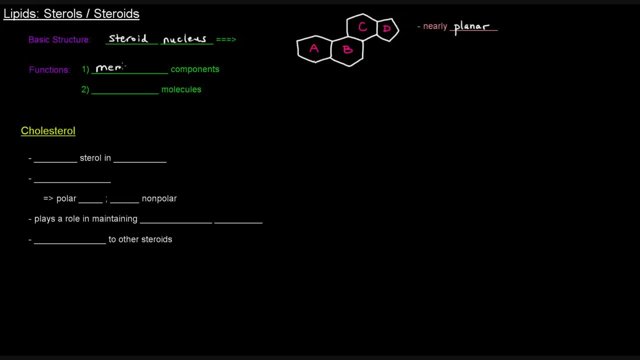 Their functions. they function as membrane components and they can also function as signaling molecules, namely hormones. The major sterol in animals is cholesterol and its structure is like this: It looks like that It is an amphipathic molecule, which means it has polar and nonpolar portions. 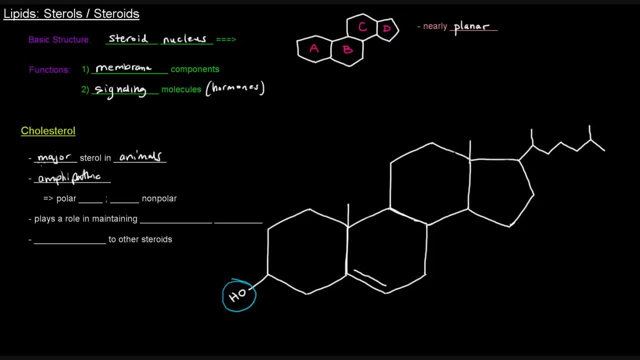 Its polar portion is actually pretty small. It's just this OH group here. It's got a polar OH. The rest of the molecule, though, is just hydrocarbons, Right Carbons and hydrogens, So the rest of it is nonpolar, which is why it can actually be a membrane component. 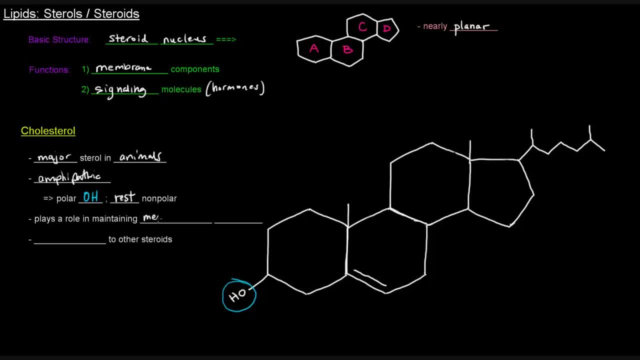 Specifically in membranes. it plays a role in maintaining membrane fluidity. So if it gets too cold and a membrane sort of begins to become more rigid, cholesterol will play a role in helping it become more fluid. And if it becomes a little bit too fluid and might break apart, it allows it to become a little bit more rigid. 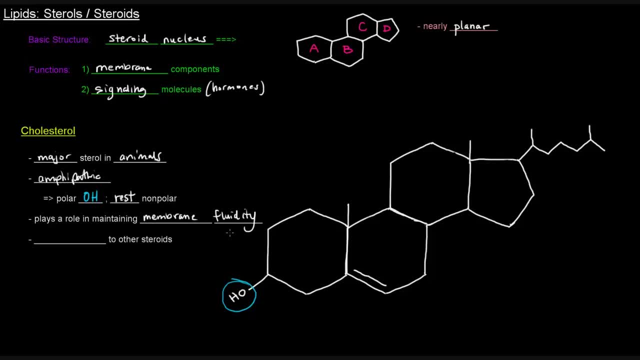 to maintain fluidity. It allows it to maintain optimal fluidity levels, So cholesterol plays an important role there. It's also important as a precursor to other steroid molecules. In fact, something that's actually pretty important to that is the numbering system of cholesterol. 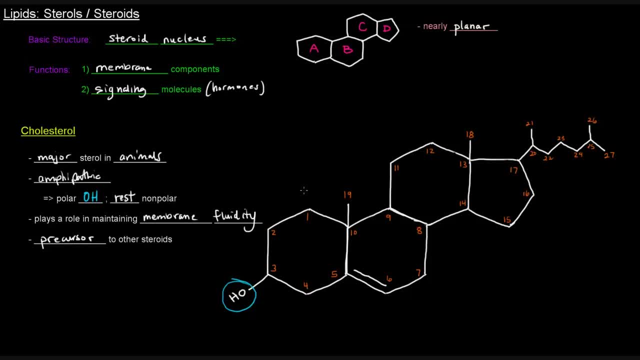 It's 27 carbons long and it's numbered like this, starting from carbon number one right there, And we go around 1, 2, 3, 4, 5, 6, 7, 8,, 9,, 10.. 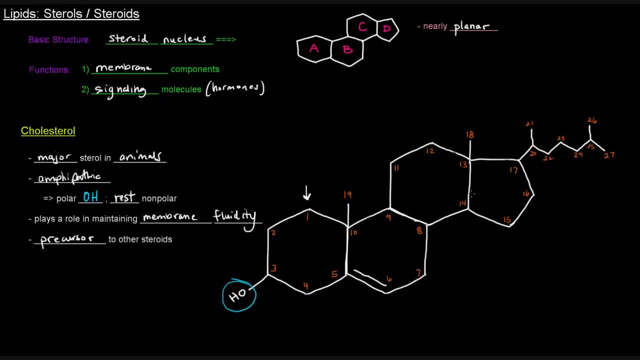 Then we jump up here to 11,, 12,, 13,, 14,, 15,, 16,, 17.. Then we jump up here to 11,, 12,, 13,, 14,, 15,, 16,, 17.. 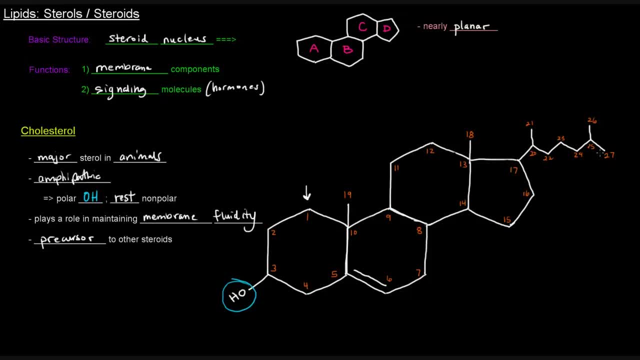 Then these two methyl groups, 18, 19,, and then 20 through 27 are on this end over here. The numbering system might not seem really important right now, but there are certain enzymes involved in sort of converting one steroid molecule to another. 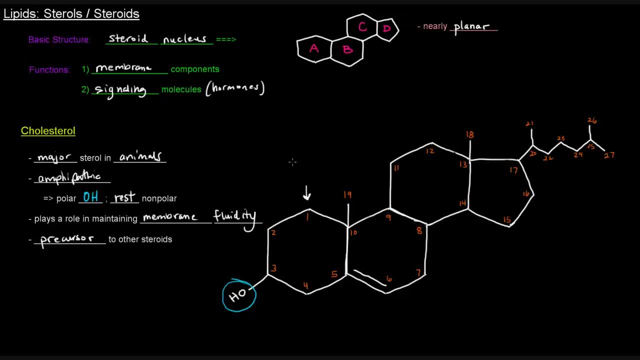 And the names of the enzymes sometimes refer to where they're actually doing whatever it is they're doing. As an example, there's an enzyme called 5-alpha reductase And what that does. that molecule is actually what takes testosterone and turns it into dihydrotestosterone or DHT. 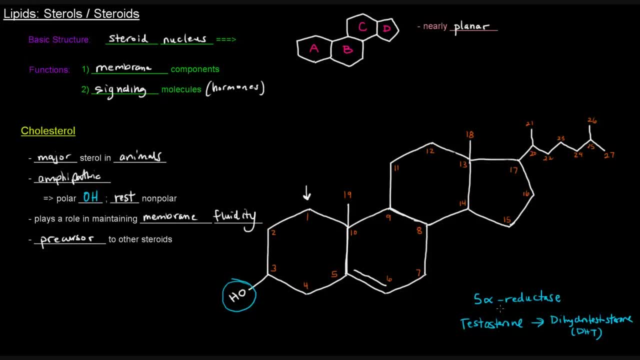 And the enzyme name 5-alpha reductase. it's actually it's reducing the 5-carbon of testosterone to become dihydrotestosterone or DHT. So that's just one example. There are other examples, but the point is that, being familiar with the numbering system of these steroids, 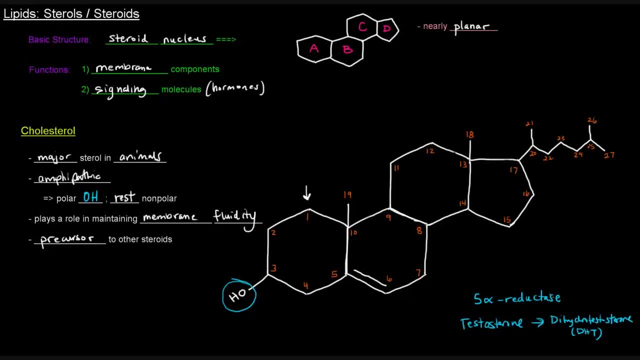 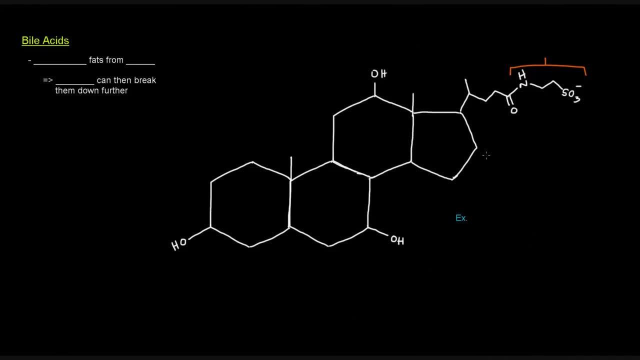 is helpful in understanding the names of the enzymes, in case you're studying those pathways. Okay, next up here, bile acids. So there are bile acids that are steroids And their function really is to emulsify fats from our diet, And what that means is basically it takes these gigantic fats that we're consuming. 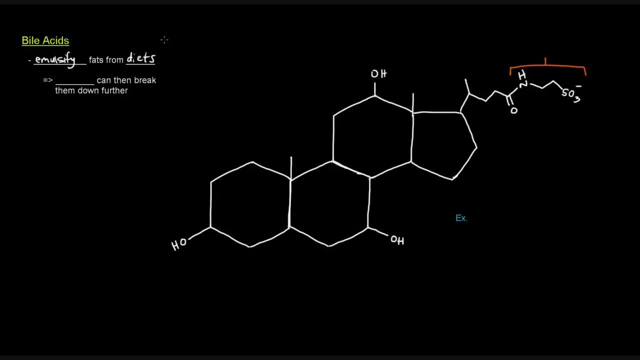 and breaks them up into little, smaller sort of molecules that lipases can act on, And lipases will go through and break down the fats further from there. So I've just drawn here an example of a specific bile acid called torocolloic acid. 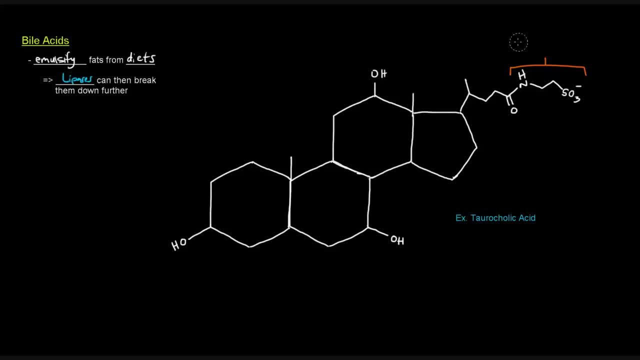 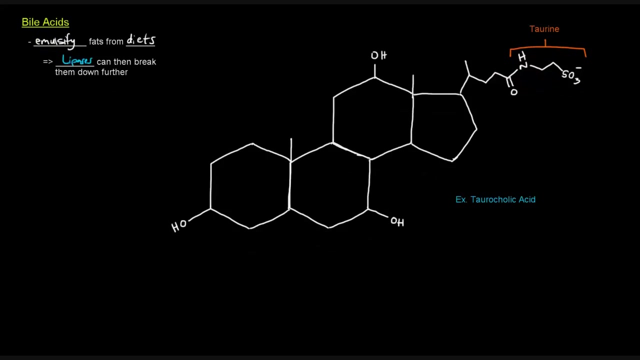 And the reason the toro portion of that name comes from this portion up here called taurine, And that taurine portion actually carries the acidic group that is carrying the negative charge after it has been deprotonated- Now steroid hormones. 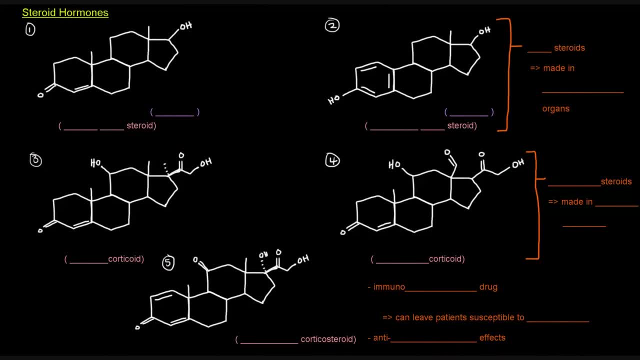 Steroid hormones. So these are the ones that I think a lot of people study. These first two up here are the sex steroids, And they are made in the reproductive organs. So over here I've drawn the male sex steroid And over here I've drawn the female sex steroid. 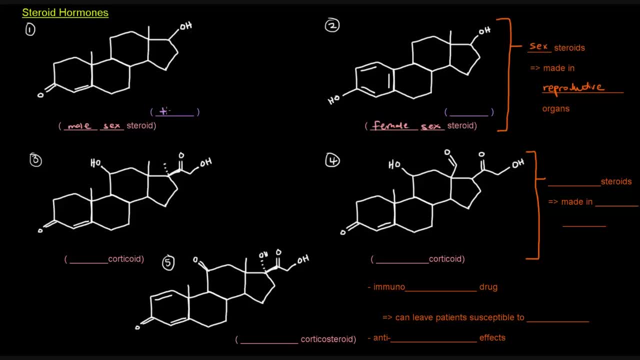 The male sex steroid is made in the male reproductive organ, which is the testes, And the female sex steroid is made in the ovaries, the female reproductive organ. So which two steroids are these? You may already have guessed it: This one is testosterone. 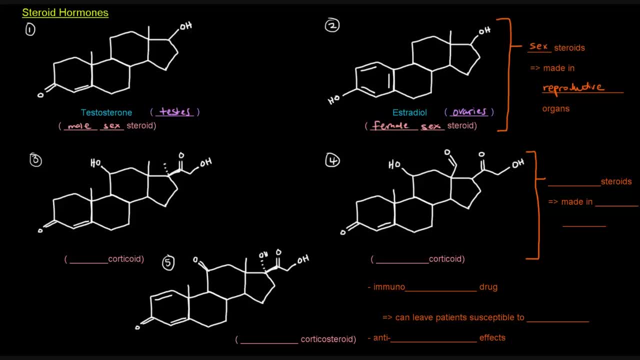 And this one is estradiol. The names can make a little bit of sense. This test refers to the fact that these things are made in the testes. Ster comes from the S-T-E-R steroid, And then O-N-E refers to ketone. 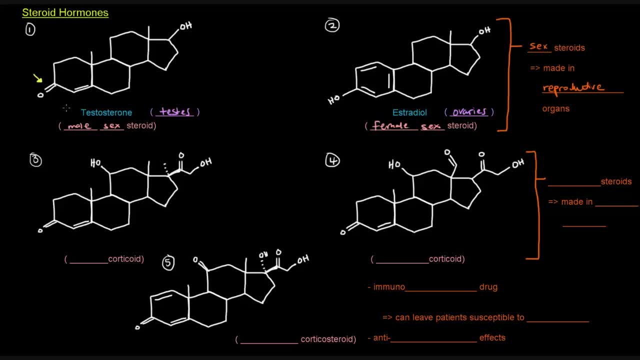 So we've got a ketone right there. So it's basically saying male sex steroid And it has a ketone in it. Estradiol- Estro refers to estrous And the diol refers to two alcohols. There's an alcohol there and an alcohol there. So these names can make a little bit of sense. They're not always surefire, But they can sometimes make a little bit of sense. Okay, next up, three and four. Three and four are the corticosteroids, Because they are made in the adrenal cortex. 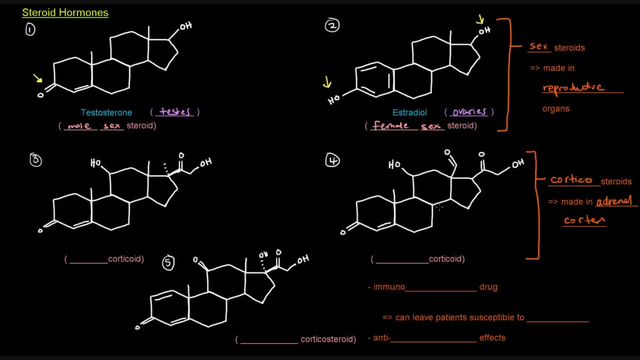 So cortex, cortico, corticosteroids- They're also called corticoids for short. The first one over here to the left is a glucocorticoid, And this one over here to the right is a mineralocorticoid. 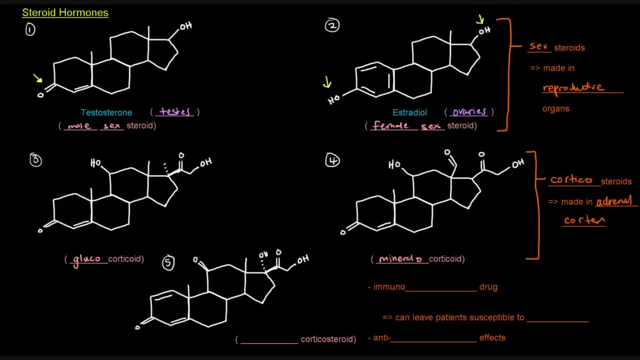 Mineralocorticoid, And you may have guessed the names of these: This one is cortisol And this one is aldosterone. Cortisol is a stress hormone, And the reason it's called a glucocorticoid is because of its effect on blood glucose levels. 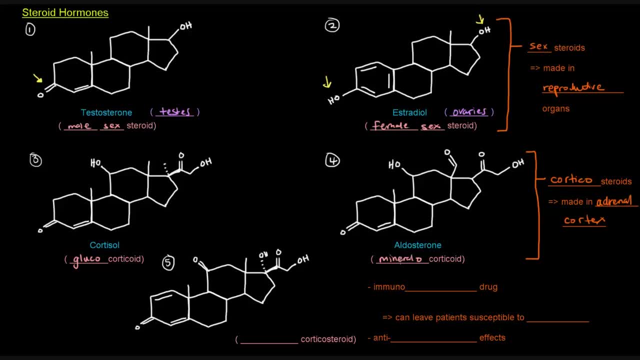 Aldosterone is a mineralocorticoid because of its effect on the minerals in our body, Specifically sodium. Sodium is a mineral And so aldosterone plays a role in sodium levels, So it's a mineralocorticoid, And the "-one"- again here the "-one"- refers to ketone. 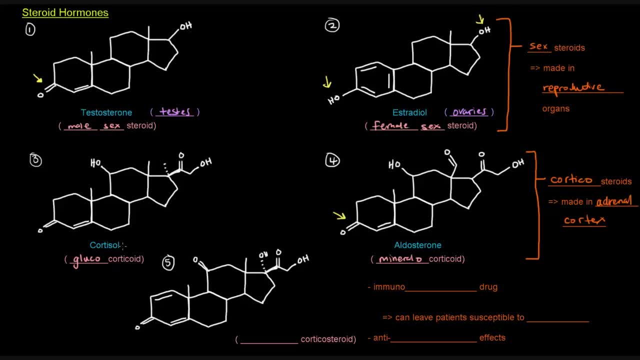 Cortisol also has a ketone, but it doesn't end in "-one" But up here it does have some alcohols, So that "-ol" might refer to these alcohols. up here Cortisol's name doesn't really lend too much to its structure. 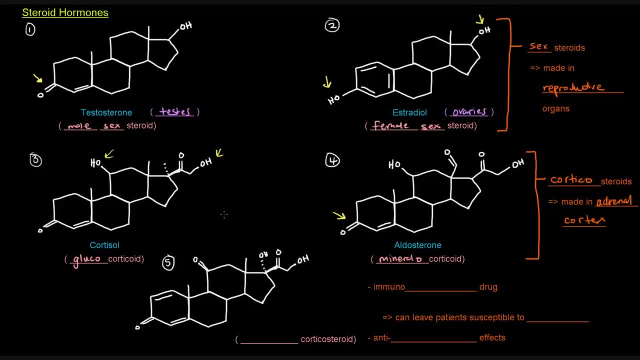 But cortisol and aldosterone are both corticoids Because they're made and released from the adrenal cortex. This last one here, number five, is a synthetic corticoid, Synthetic corticosteroid, Synthetic corticosteroid, And it's actually called prednisone. So prednisone is used to treat anti-inflammatory diseases- Anti-inflammatory diseases- And it is an immunosuppressant drug. So, though it can treat anti-inflammatory diseases, because of its immunosuppressive effects it can leave patients susceptible to infections. 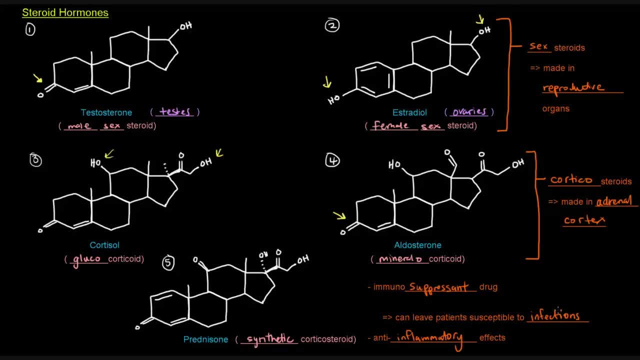 So I don't know. I'm just as soon as I heard that, I thought: okay, so if someone is taking prednisone for some sort of disease, we might want to make sure that. you know, we make sure that everything that we give them is pretty clean. 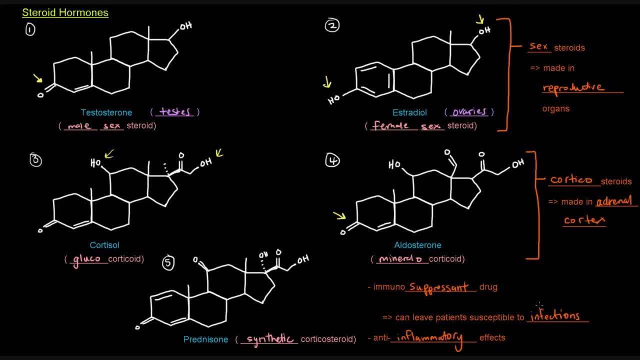 and free from infections, Because they're especially susceptible to infections. Now, all these steroid hormones can, basically are important in signaling. So because they are steroid hormones, they can. they will somehow make their way to the nucleus of a cell.